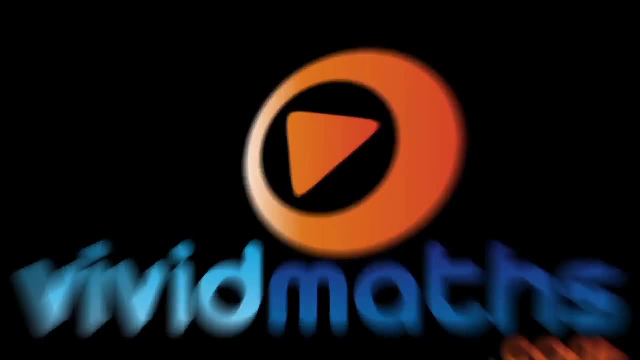 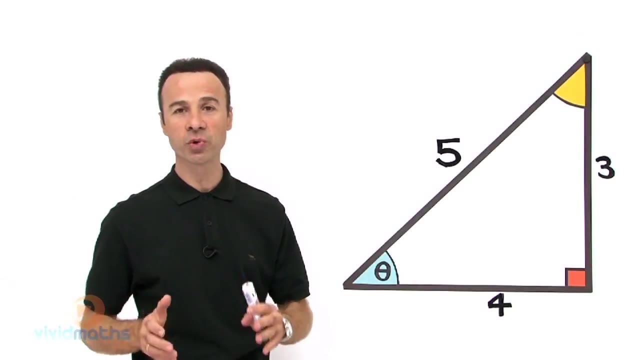 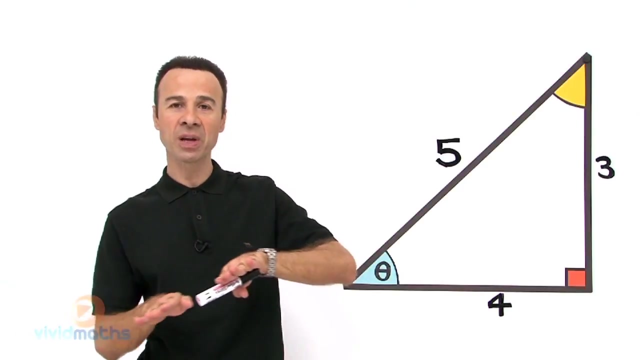 Hi guys, we are working with trig ratios and I am going to work with one word. it is called contrast. What does contrast mean? It is when you take two opposites and you put them next to each other and you contrast them, or you show the differences You can highlight and 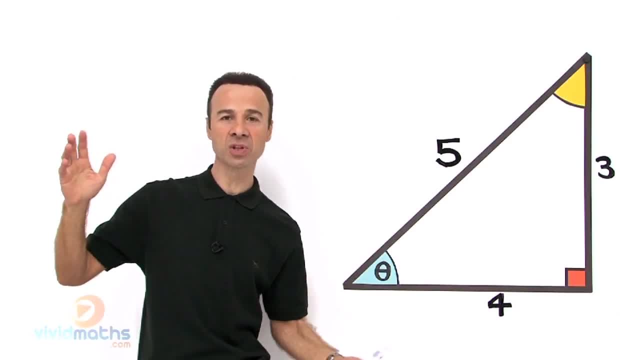 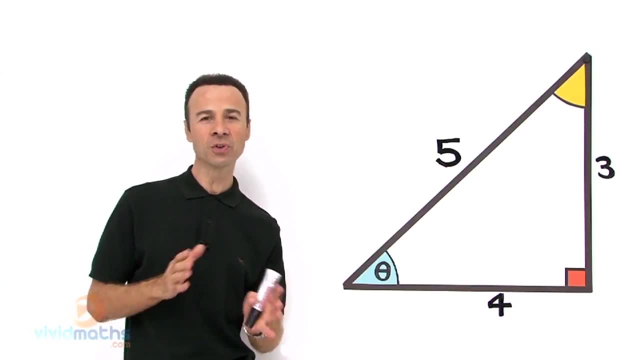 dramatize an idea. If you want to show how tall something is, you put something short next to it. So you get opposites and you put them together. Well, there is two opposites here, called sign and cause. Well, they got different type of angle systems and what I 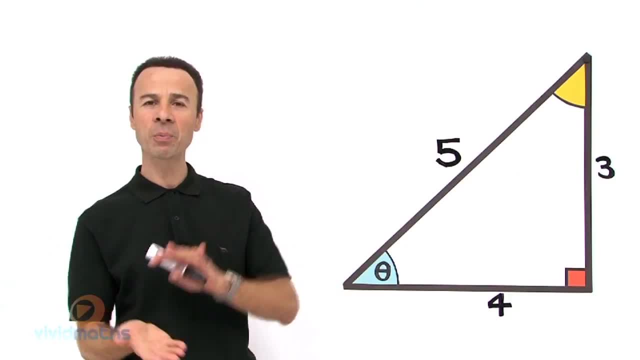 am going to do is show you how you can have these two guys and come up with the same answer on a ratio. So let us use this example here. right next to me We have a right angled triangle. There is a little right angle down there, a little friend there he is, And we got angles. 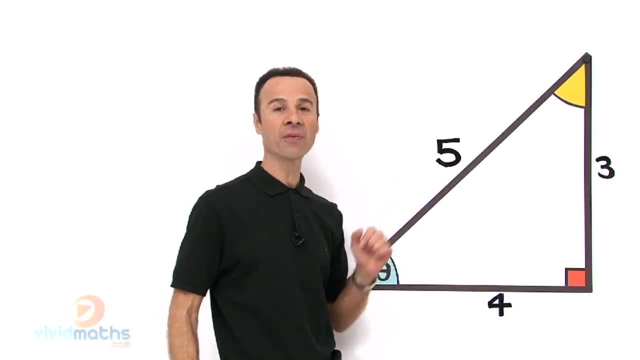 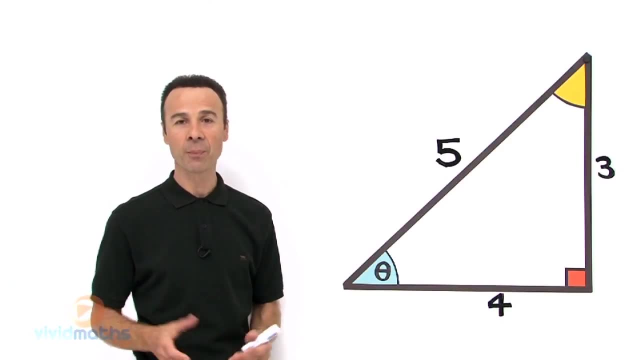 around this and we got lengths. Now the lengths we have is 5 for the hypotenuse. over here we have 3, and over here we have 2.. Over here, down the bottom on this length, we have 4.. Now what the question ask is to find: 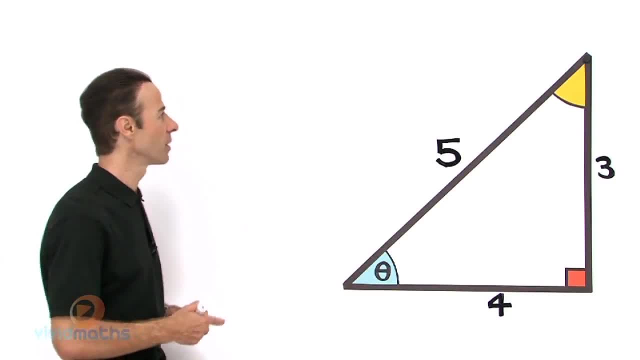 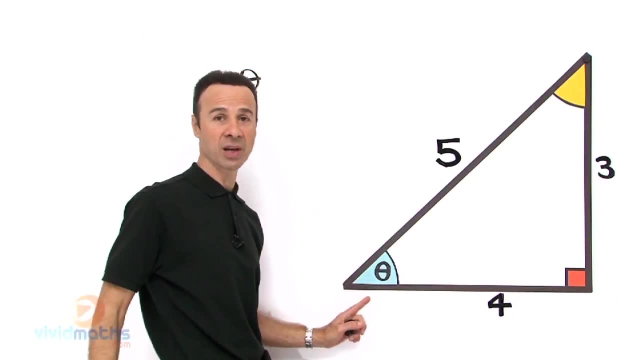 sine theta as a ratio. So if we are looking for sine theta, quite simply what we do is we write down sine theta, which is this guy down here. So we are working with this angle: Sine theta equals. now what does sine theta equal? again, It is opposite over what Opposite. 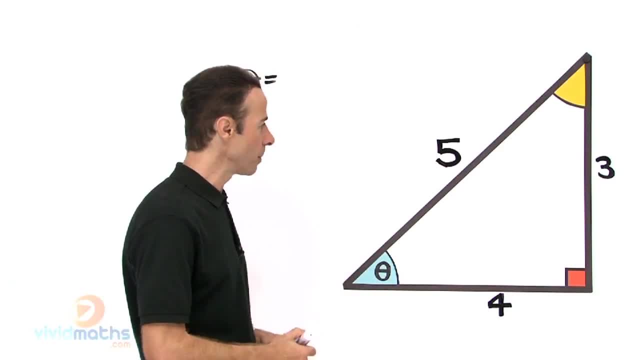 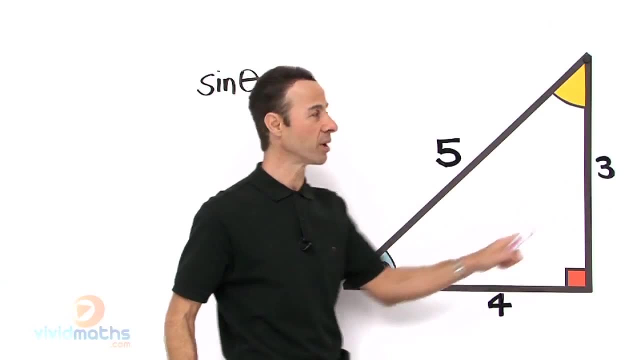 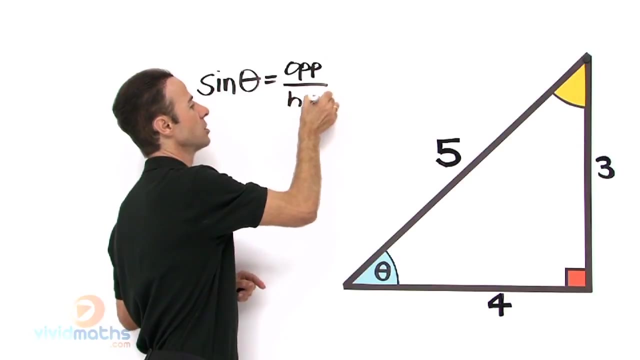 over hypotenuse. Now, if we look at this and we want to find opposite, it is straight ahead, isn't it Like that? So straight opposite the sine theta, pointing right across there is the number 3.. So let us write down first of all: opposite over hypotenuse. So let us go back to that again. Opposite- 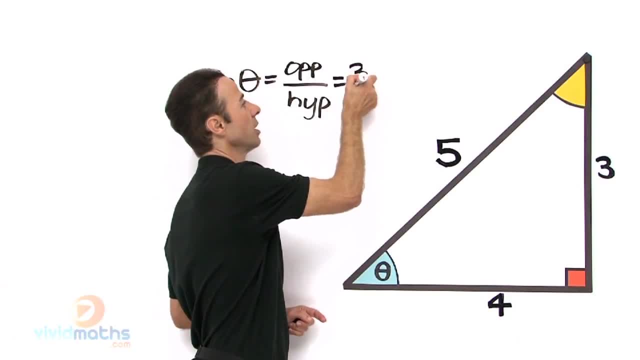 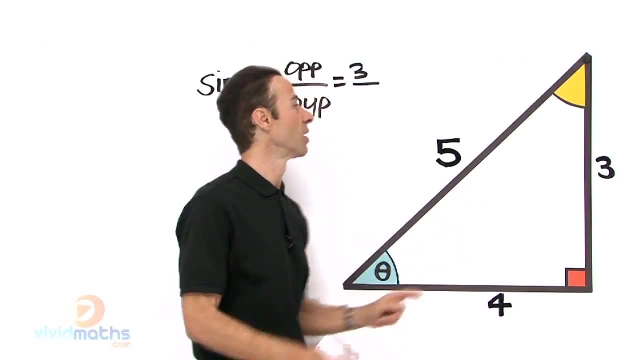 is 3, so let us write down 3.. So that is 3 over. now, over what Hypotenuse? yeah, It says hypotenuse, So hypotenuse here is 5.. So sine theta, quite simply, is 3 fifths. yeah. 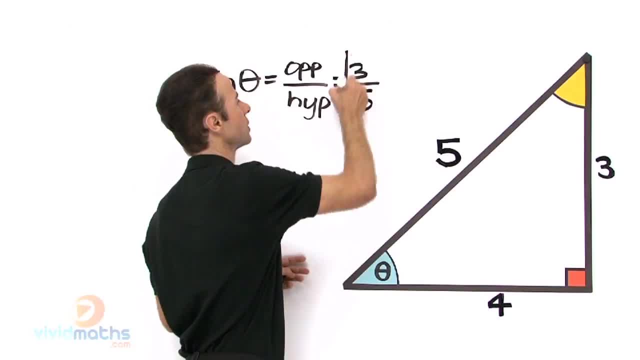 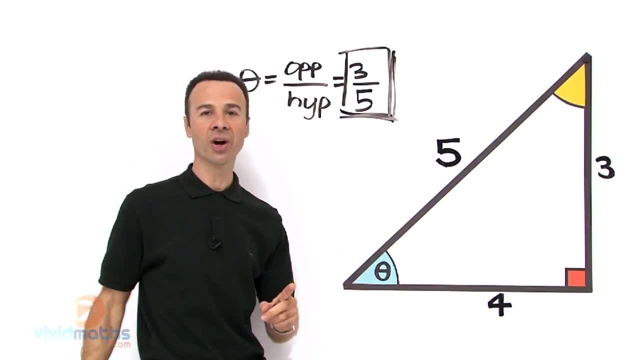 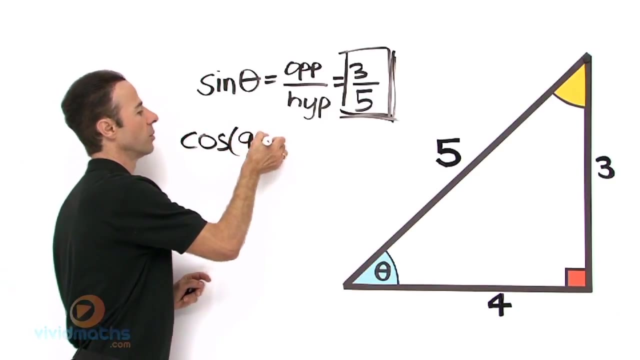 So sine theta is 3 fifths. So there is our 3 fifths. Now what we are looking for is cos 90 minus theta. for the second part of this question, Let us look at that now. looking for cos bracket 90 minus. 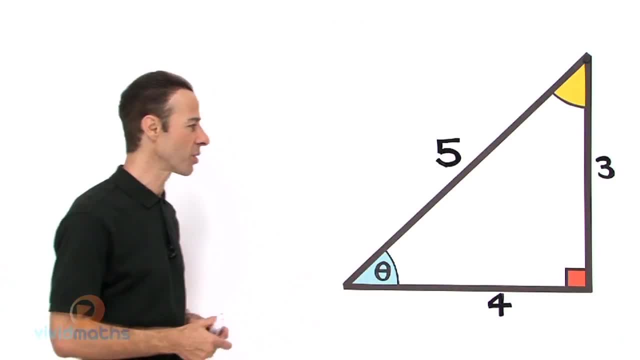 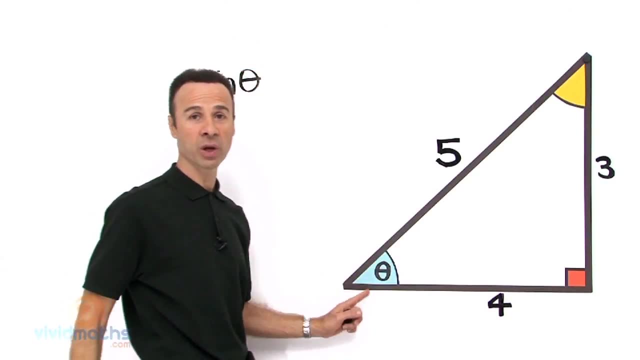 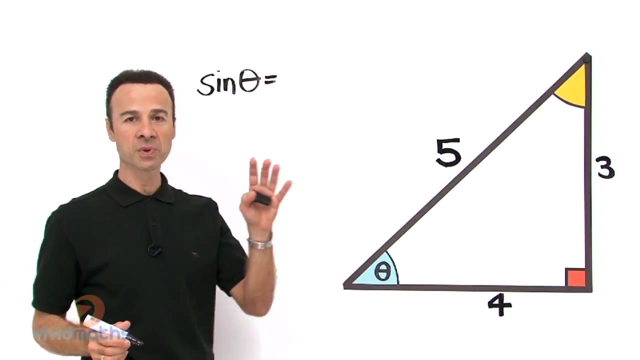 to find sin theta as a ratio. So if we are looking for sin theta, quite simply what we do is we write down sin theta, which is this guy down here. so we are working with this angle, sin theta equals. now what does sin theta equal? again, It is opposite over what Opposite. 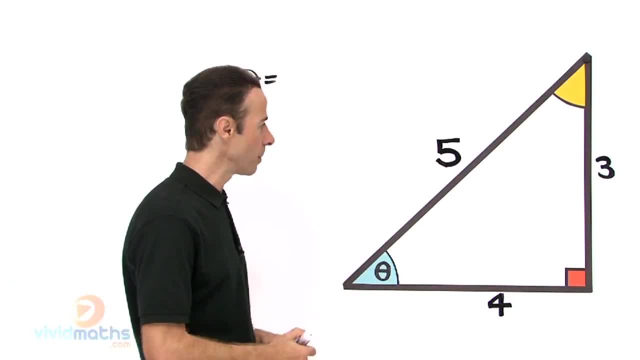 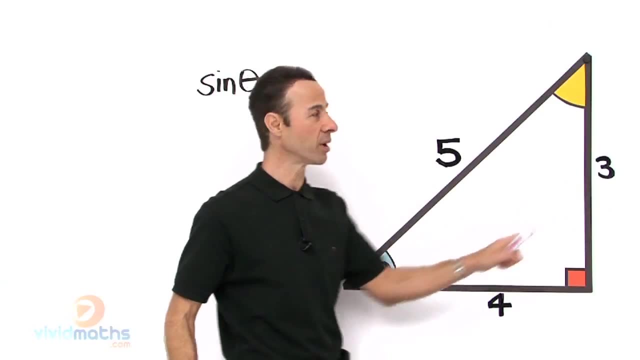 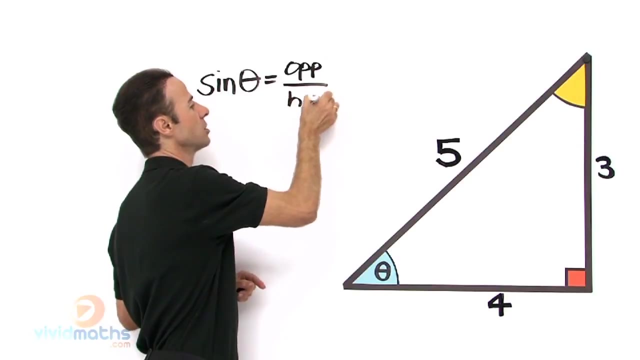 over hypotenuse. Now, if we look at this and we want to find opposite, it is straight ahead, isn't it Like that? So straight opposite the sin theta, pointing right across there is the number three. So let us write down first of all: opposite over hypotenuse. so let us go back to that again. 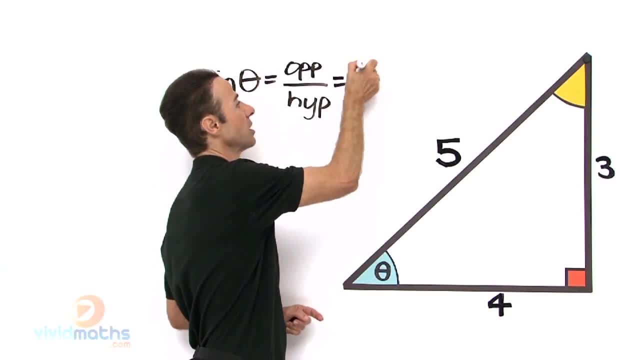 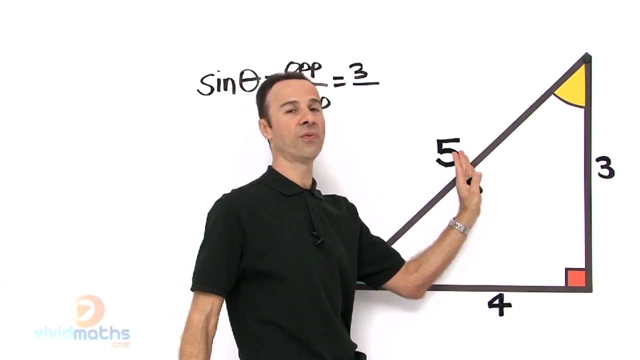 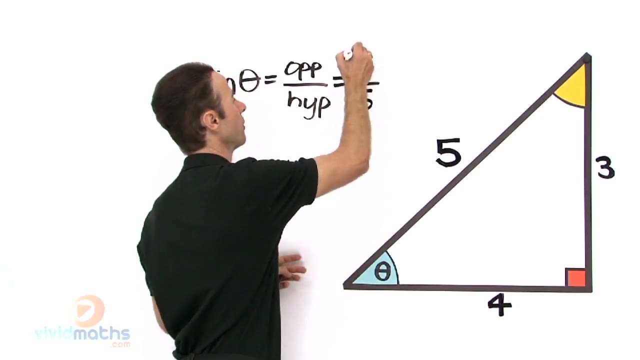 opposite is three, so let us write down three. So that is three. over now, over what Hypotenuse? yeah, it says hypotenuse, so hypotenuse here is five. so sin theta, quite simply, is three-fifths. top of the hypotenuse here is three-fifths. So there are three-fifths what we are looking. 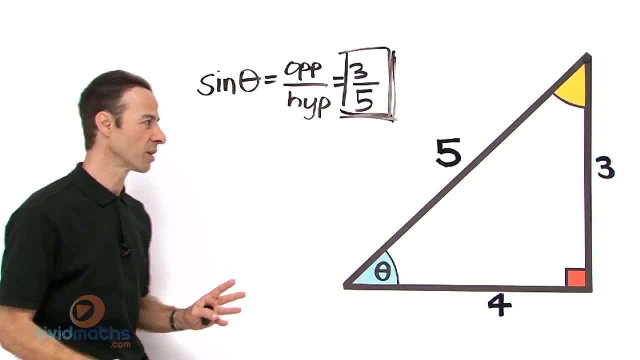 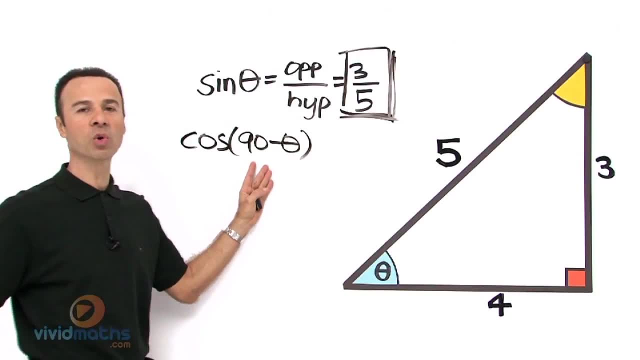 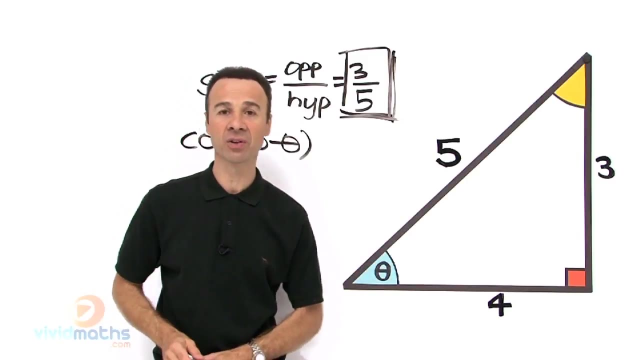 for is cos 90-theta. for the second part of this question, let us look at that now. Looking for cos Now, if you have never come across this, I am going to show you how to He understand the strategy involve to you. Cos 90-theta clearly is not in our diagram, is it You? 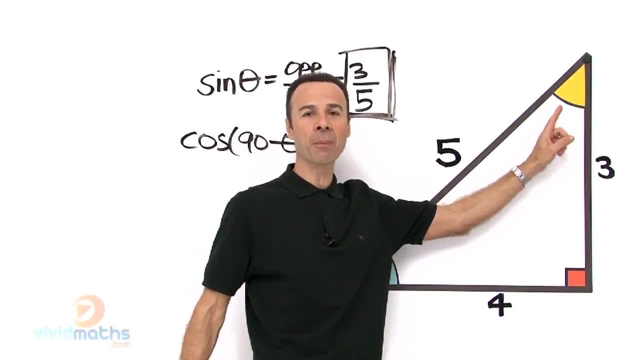 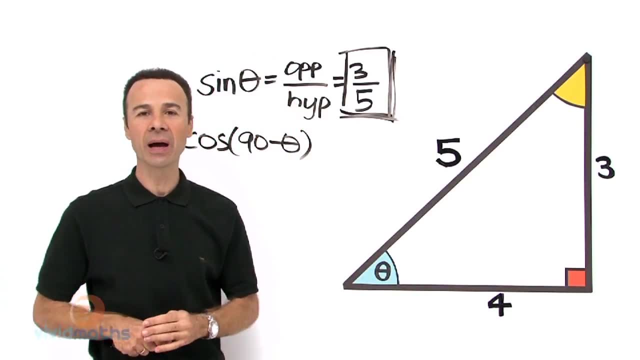 cannot see it anywhere in the triangle. we have theta here, We have kind of empty angle angle up here, so I am going to work it out up here. Now, what is 90 minus theta exactly? Well, it works like this. you know how all angles add up to 180 degrees in a triangle. 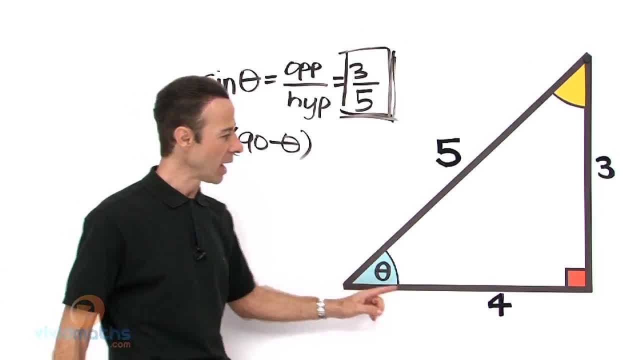 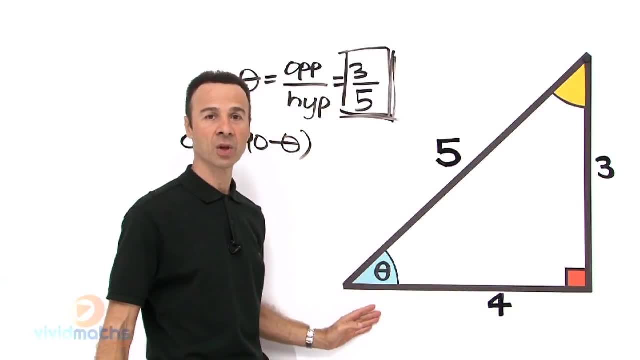 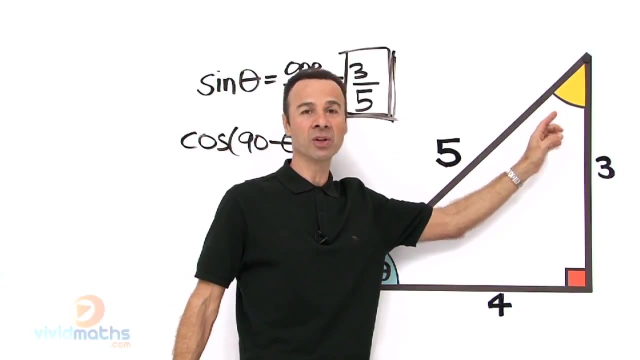 Well, if we have theta here, no matter what it may be, if we have theta here and we got 90 here, whatever is left clearly has to be 90 minus theta. Whatever that angle is, take away that whatever is left is going to give us that. So this angle here will be 90 minus. 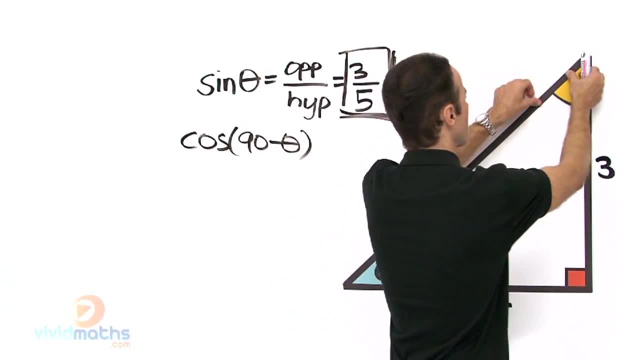 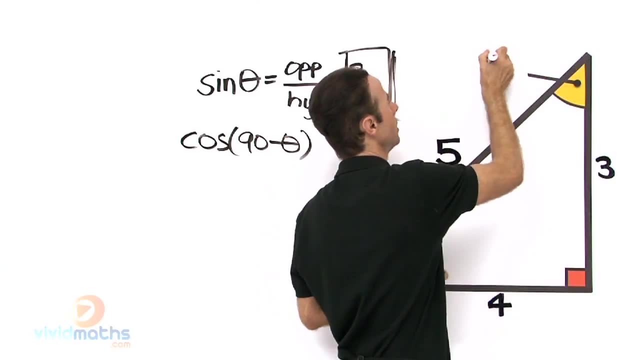 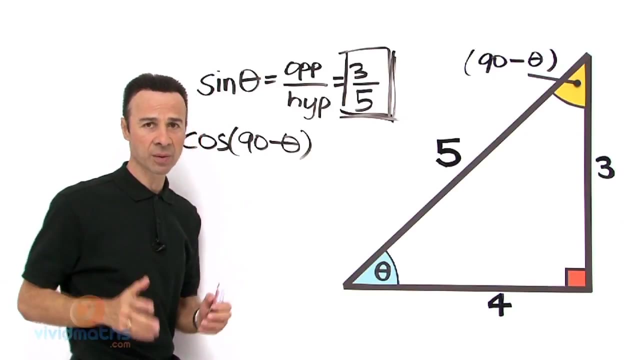 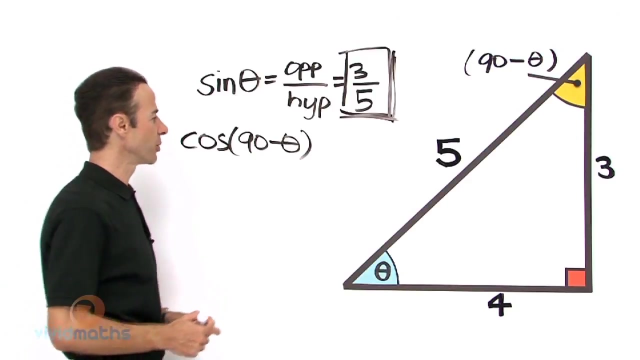 theta. So let me just put that in: I have 90 minus theta. now that is the angle in there, cause angle sum of triangles. I explained. So if that is 90 minus theta, we are looking for cos 90 minus theta. I wonder what that is going to equal. So first of all, what cos? 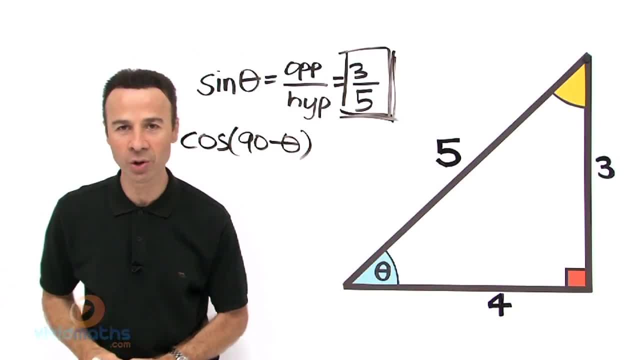 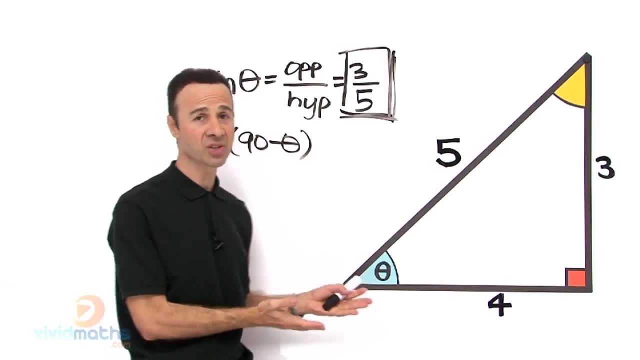 theta. Now, if you have never come across this, I am going to show you how to understand the strategy involved here. Cos 90 minus theta clearly is not in our diagram, is it? You can not see it anywhere in the triangle. we have theta. here we have kind of an empty angle. 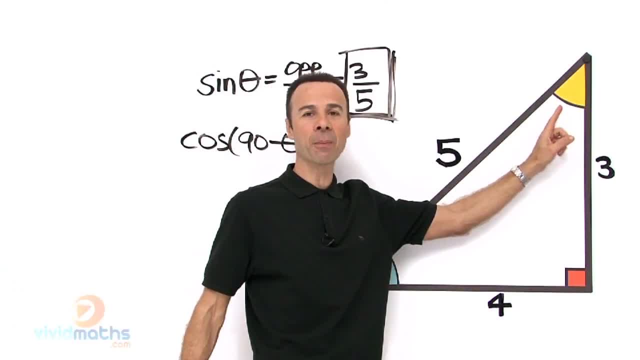 Now, if you have never come across this, I am going to show you how to understand the strategy involved here. Cos 90 minus theta clearly is not in our diagram, is it? You can not see angle up here, so I am going to work it out up here Now. what is 90 minus theta exactly? 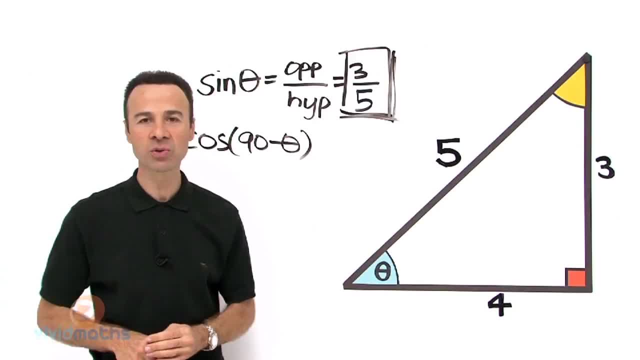 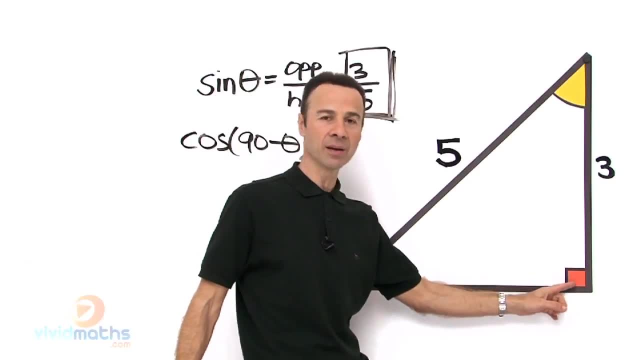 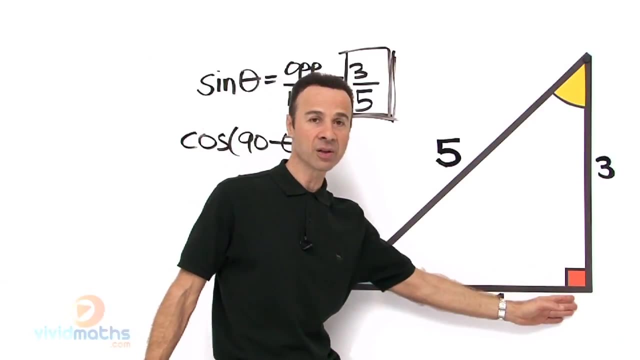 Well, it works like this. you know how all angles add up to 180 degrees in a triangle. Well, if we have theta here, no matter what it may be, if we have theta here and we got 90 here, whatever is left clearly has to be 90 minus theta, Whatever that angle is take. 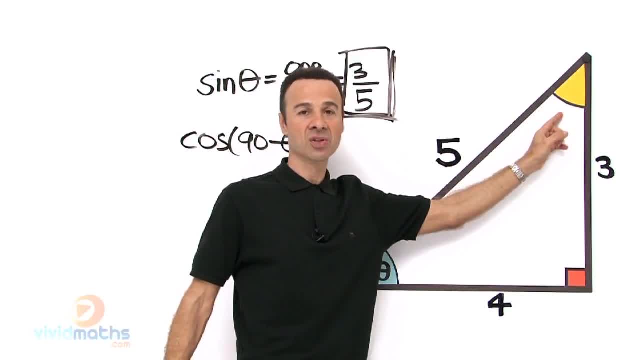 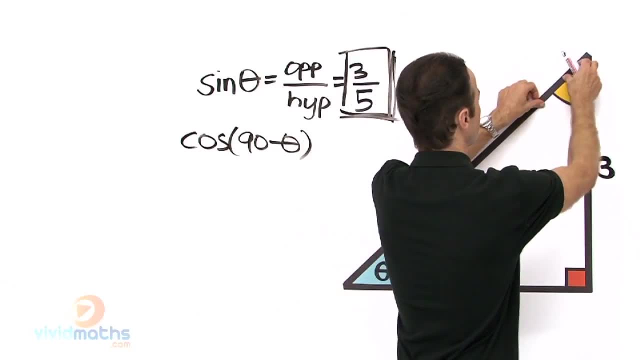 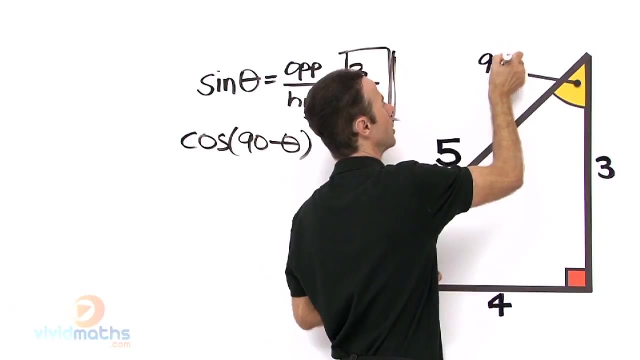 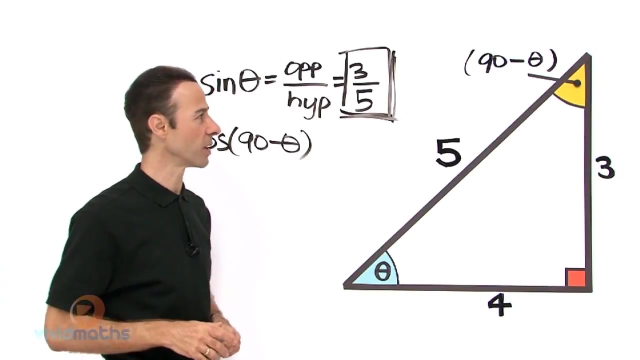 away that whatever is left is going to give us that. So this angle here will be 90 minus theta. so let me just put that in: 90 minus theta. Now that is the angle in there, because angle sum of triangle, as I explained. So that is 90 minus theta. we are looking for cos 90. 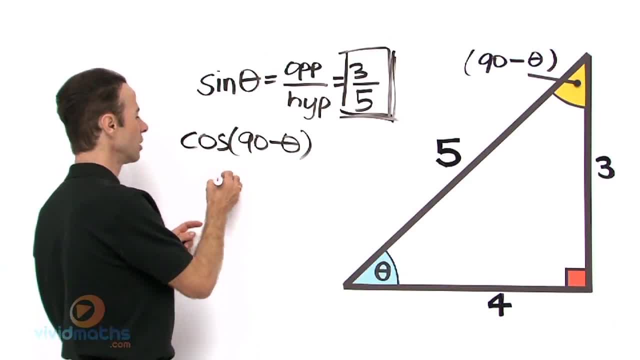 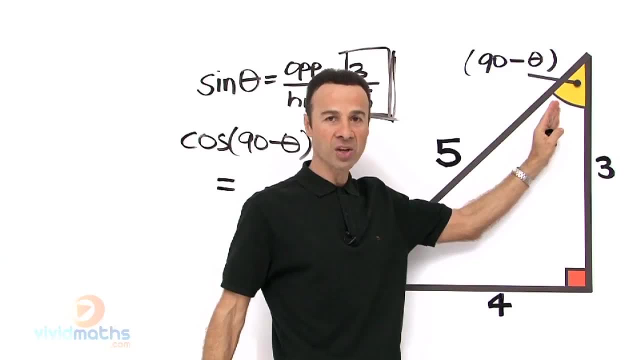 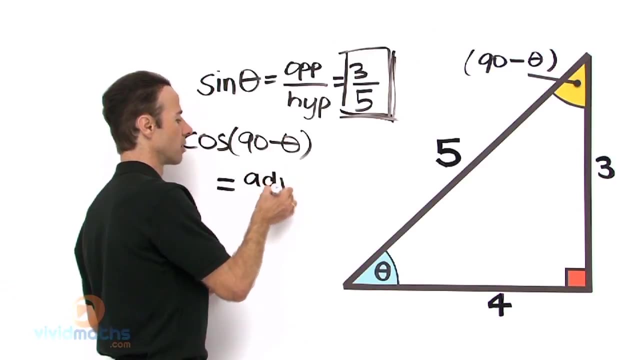 minus theta. I wonder what that is going to equal. so, first of all, what does cos equal? Cos equals adjacent, isn't it whatever adjacent is to the angle. So if we are looking for cos of this angle, we got adjacent, which happens to be 3 again, doesn't it? So let us write down: adjacent, adjacent over. 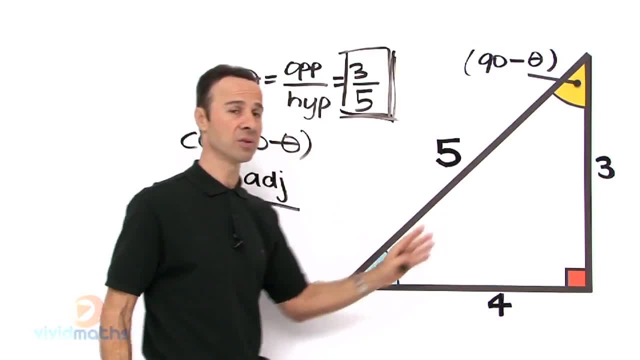 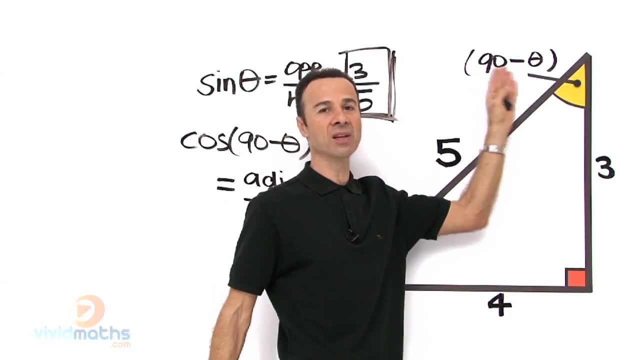 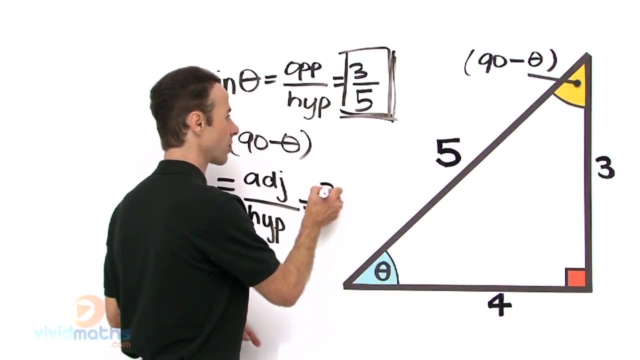 adjacent over? what Cos is adjacent over hypotenuse over hypotenuse? let us see what that equals: adjacent for cos 90 minus theta, so that is a cos now. so going down, adjacent is to the left, there right, So it is 3. so that equals 3 over hypotenuse over 5. so clearly what we. 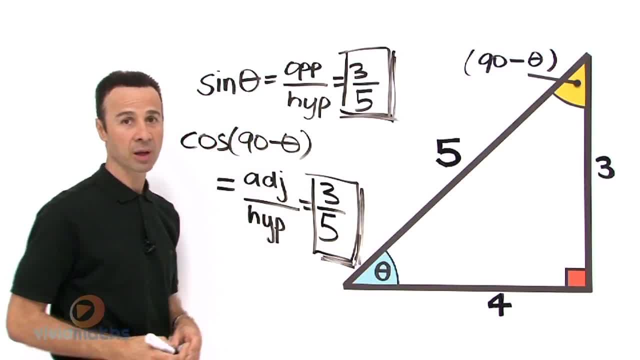 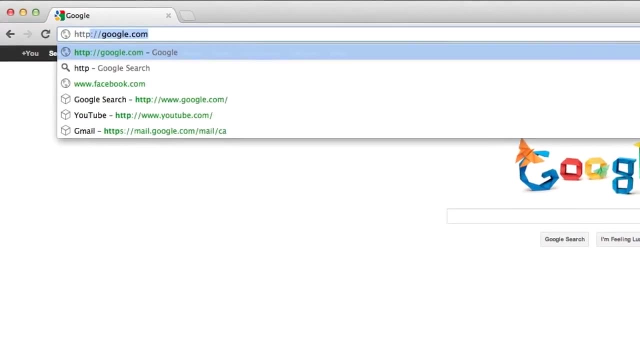 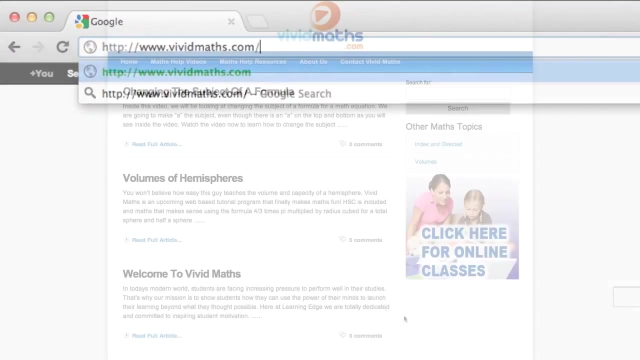 have here is two contrasts: cos with sin- and both come up with exactly the same answer: sin theta is 3 fifths and cos 90 minus theta is also 3 fifths. Thank you for watching. If you enjoyed this video, make sure to hit the like button and.